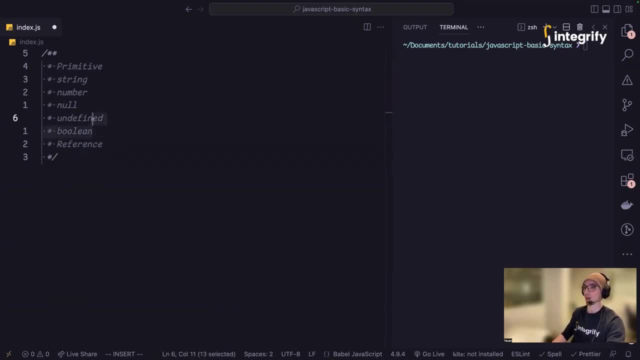 but let's just focus on the on these five, most five use points. And then in the reference we have this, A different one here. So in the reference it's an object. That's the only one in the reference. you might be wondering where's the array, Where's the functions? So all of those are. 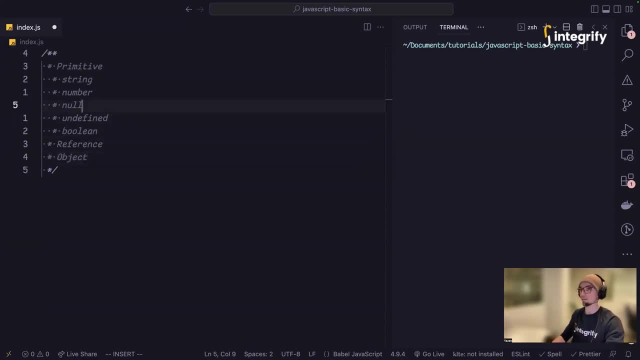 actually objects at the end of the day. So what is the big difference between the primitive and reference? So I can just talk about that just briefly. So the kind of the big differences between the number and an object or a reference is that when you, for example, in comparison, 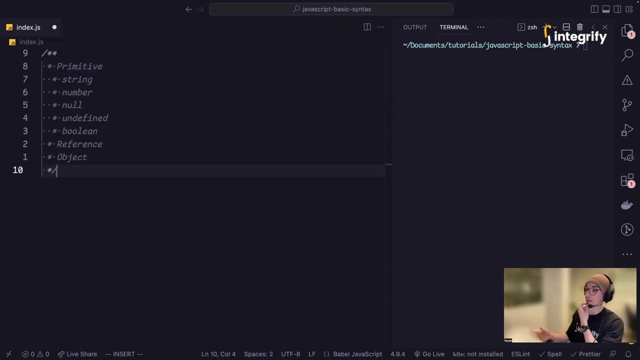 when you compare two values or when you copy a value. so the when it comes to primitives, it copies by its value, But when it's referenced, it copies by the reference where it's located in the memory. we can definitely talk about that in more details And so on in the next videos, but let's just just keep this rolling. 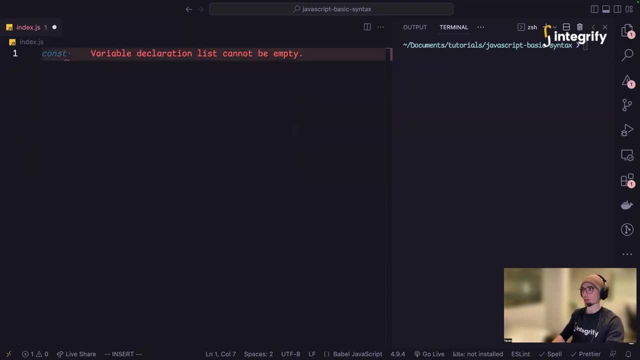 Alright, so let's start with the most, or the first one is variables. How do you declare variables in JavaScript? So we have the very old ways. was using very far, for example, bar name well, by John, but but for this is, it has so many like bad things. 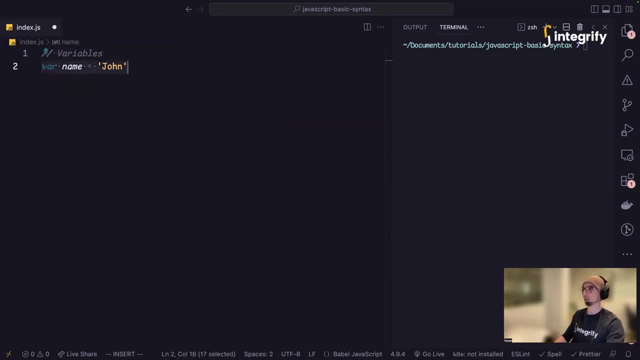 disadvantages, which it's not really the best thing to do, which I'm not going really to go and give an example there or talk about it, So, but I will tell you: just stay away from bar. So it's better for you to go with the ESH syntax, So with the let endpoint cost. so let's start with let. So 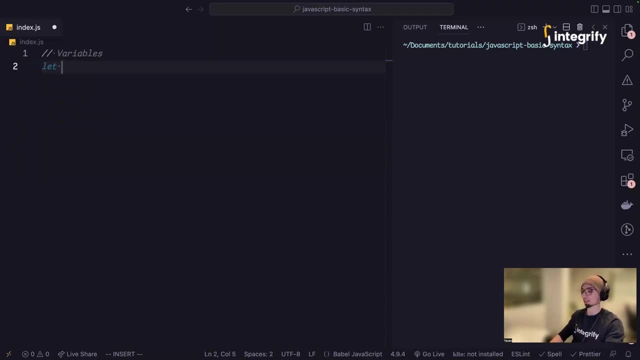 it. so, uh, what's what's good about late is that you would basically, uh, if you have a variable that is that is that has a that has initial value, and you would, you would like to change it, uh, later on. so, uh, then, then this is: this is a good place, or this is a good time for you to use a late, so in the 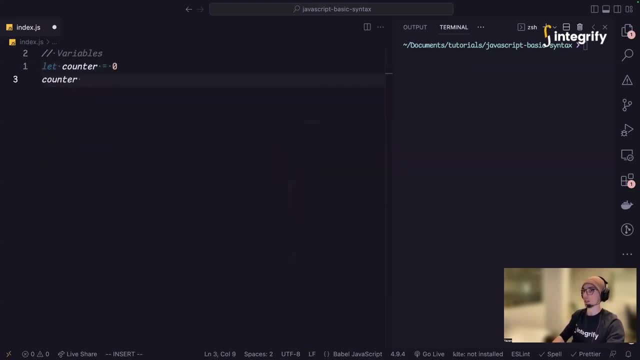 case, in this case, here that we are, we can just initialize and and assign a zero to a counter and then later on we could say, okay, go ahead and and add one to the counter. so if i at this point just consolelog counter: uh, let's just have a table, fix the table, uh, save, like just run the. 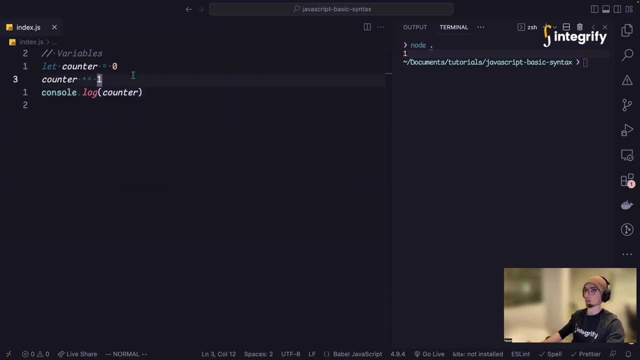 program. you see that we have number one here printed. uh, if i uh, i just maybe add five to it and save. we run it again and you see now we have six. so it's basically kind of uh, you, uh in it you can uh, you can reassign the value. but what's what's really good about it that? 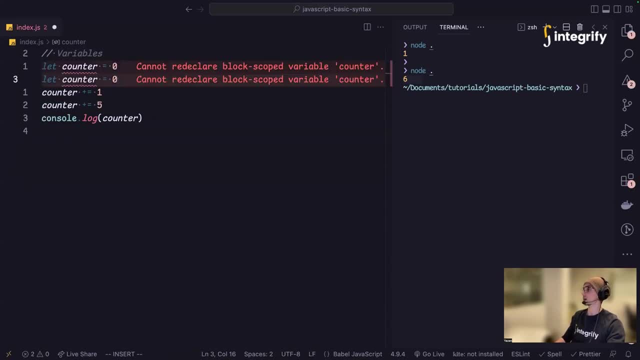 yes, you can reassign the value, but you cannot, uh declare an another variable with the same name in the same scope. uh, so for, for example, for scopes, uh, let's, for example, just have a, for example, a function, uh like count, for example, and then we, we are free to name counter here. 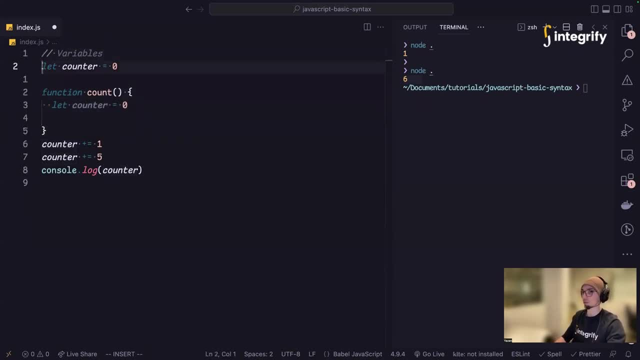 it's not going to throw an error because they live in two different scopes. here it lives on the global scope and this flip counter lives in the uh, in this underscore, uh. so that's what i'm good about about it: uh, it's mostly, mostly scope based, uh. so next time, next. 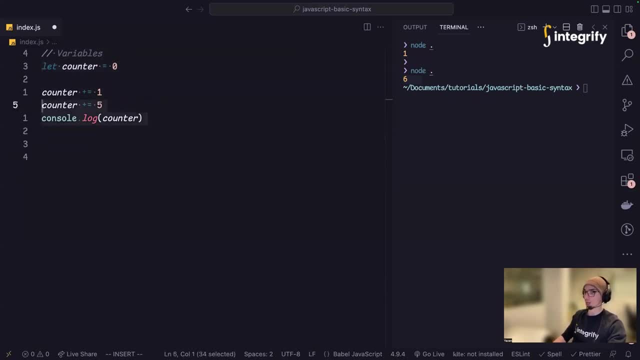 next thing is here: what if i want to uh create a variable and basically never change its value? so here comes the cost: uh, const is uh, it's basically a variable, that uh, or a way that you're declare a variable and and no matter what you do, you are not allowed to change it, like, for example: 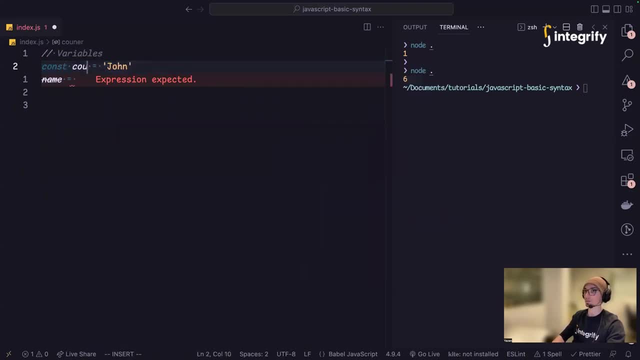 if i would go with counter again, uh, with the same variable, and i'll say the counter is one i cannot do, plus minus one here, uh, this one here, yeah, uh, let me just go ahead and console the log counter, let's see what we are going to get. and if i press it, uh, we get a type error assignment. 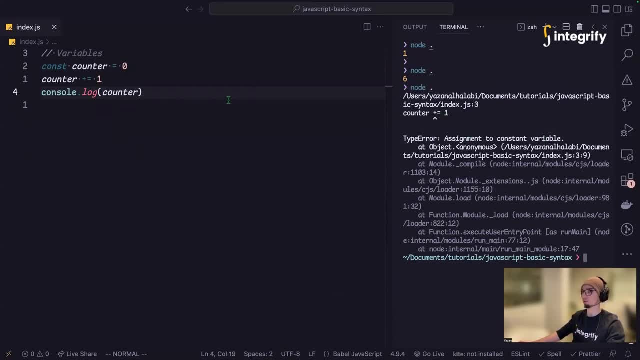 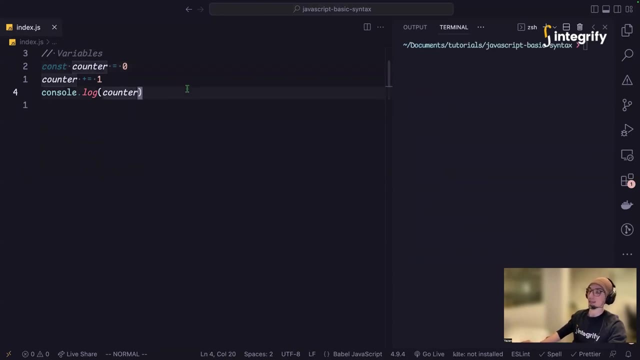 or constant variable at that position. so we cannot really uh reassign values to go on. so, uh, now here, like, if you wanna- now you're wondering maybe, hey, which one i should choose, like personally, what i, what i go with, i go with, uh, with cons, to be at that as a default, uh, default. 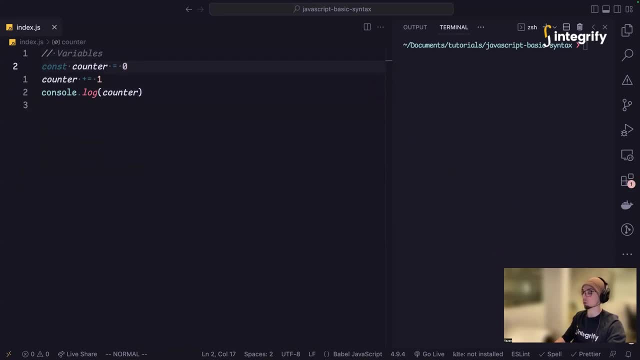 way of doing it, or depending variables, and in case i want to, uh, i would like to uh create a variable that that change later on, then i would. i would probably go with it, but by default i would go with noise. uh, you might have your own personal preferences. it's up to you and this is there is. 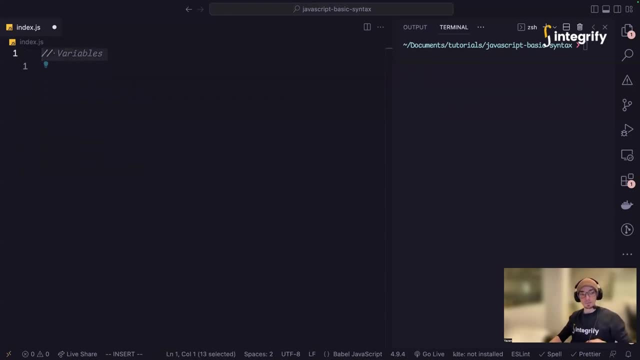 not that big of a difference. that's more about personal preferences here. uh, yeah, so, uh, so that's about. that's about variables, uh, let's. let's now jump into the- uh, the big data types. so we talked about, like at least six, uh seven data types. we're going to talk about five of these, so, uh, we're. 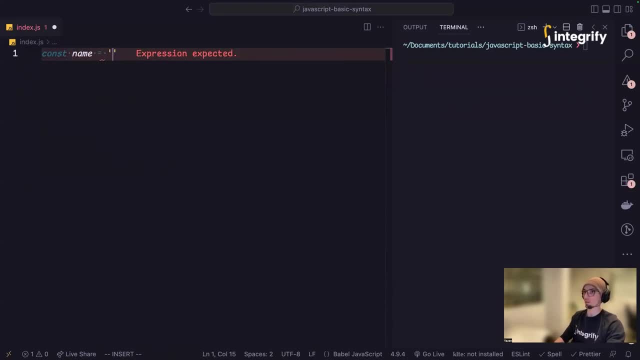 starting with the, with the strings, so we can have a variable here, uh as an in. so this is how to create: uh, create a value, a string, a type string and assign it to a variable. we do have another type, which is an age, for example. here's the number and the other ones we talked about is the. 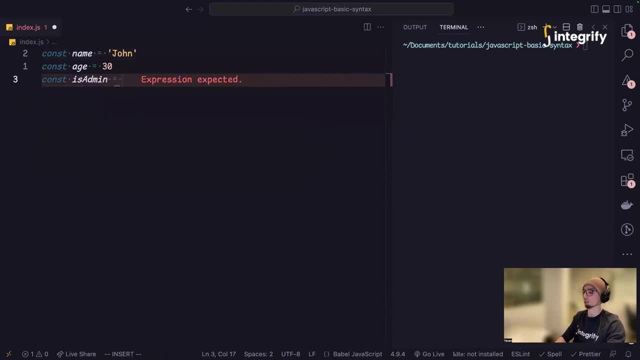 boolean type. so, for example, if you have a value that you're going to check whether, uh like, it's more like a logical way or or uh kind of, yeah, a comparison. uh, for example, you are checking, hey, is this user who's signing in or who's trying to access our- uh, this page? 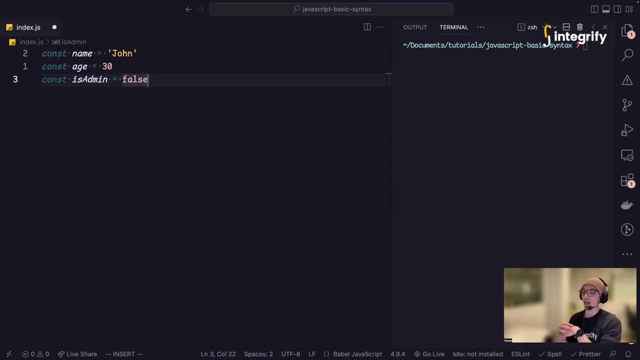 is he an admin or not? so most of the cases, uh, the, the data type of that specific kind of variable would be an or a boolean. so, whether true or false, that's, there's no. third, uh, there's option there. uh, the other one that i tried we talked about is, as well, like undefined. maybe you have a student. 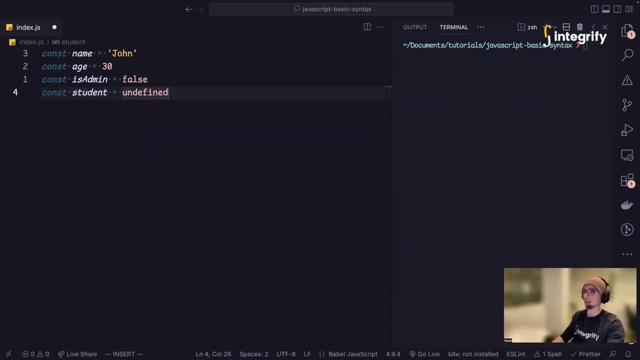 and you don't really have a. you don't really have a a value for it yet, uh, but maybe you would assign a little something- Yeah, value- later on. that's one as well, as you have, for example, another, another data type which is null. so the difference between undefined and null is that null like this: it's there, but it's empty. 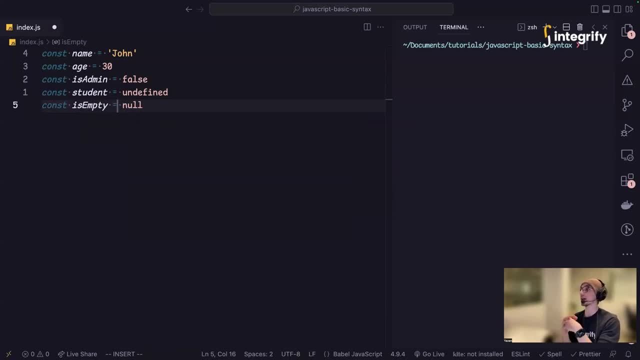 you can kind of think of it that way, but undefined, it's not there at all. that's kind of the two main keys or two main differences here. so what's next? let's talk about, maybe, objects. so if you want to create an object- so, for example, let's call this red- you create it with all we have. let me just 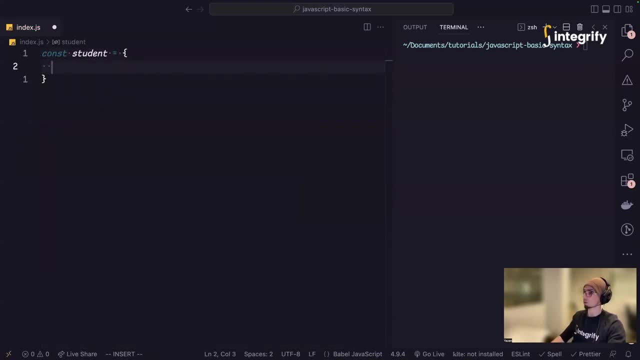 remove all these and leave just this one. so you want to kind of hold. or let's talk about like: what is an object? so object is it's just a data structure and you could think of it as maybe if you're from another other other program, as a collection, so you have a key and a value there. so, for example, what is the name, a key and 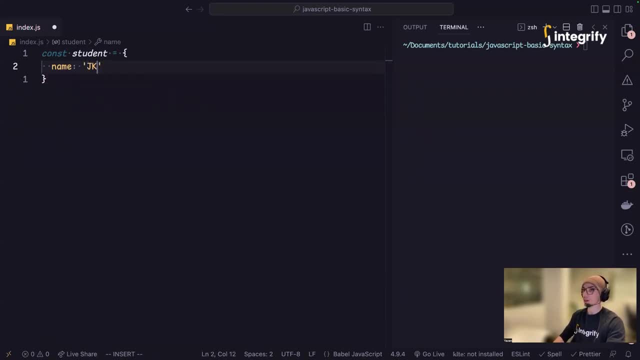 a value. so the key could be basically anything. it could be a, a name, or not necessarily everything, only, i guess, only two kind of types. so a name, a string or what, or a number, maybe it could be something like that. it doesn't matter. so that's a key, a value, on the other hand, it could be any. 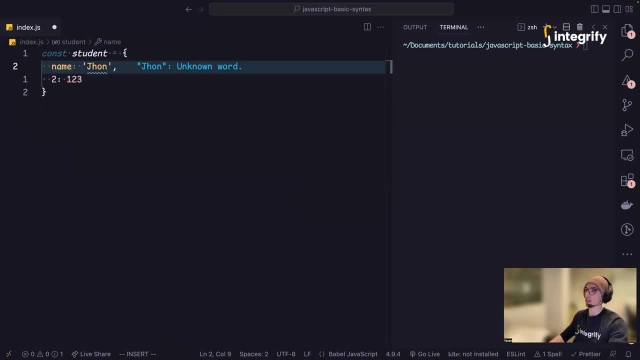 of the data types that javascript has. so you could say anything, anything very likely. so we call this part as p and the other one adds value and, uh, the whole entire thing. like, what is this name? yeah, it's a code of property. uh, but the uh, the moment, the moment you have a function, for example, as a, as a. 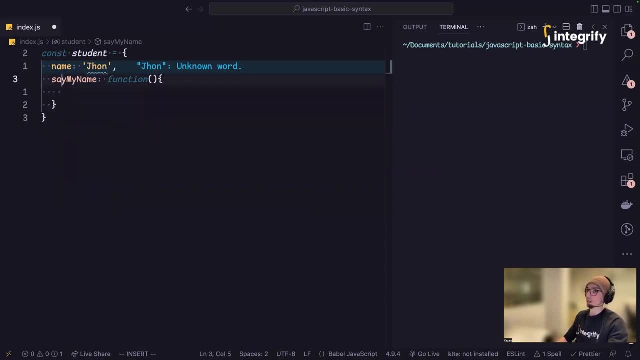 value for that key. uh. then what do we call this? we call this a, a method, uh. so, for example, you could say: uh, maybe return uh this dot name. so this, in this case, it refers to this: uh, object, uh, and we have a name property here. it's called: uh john, i think there is a type of here, let's join, uh, so. 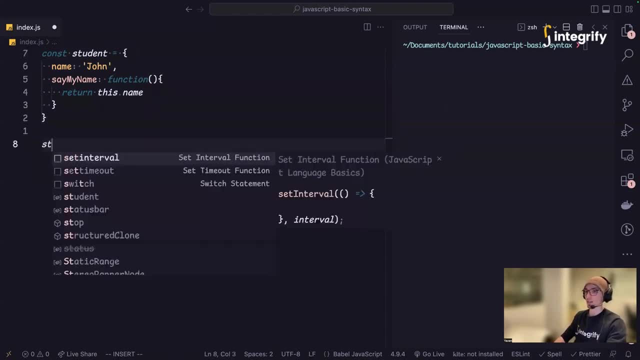 let's. let's see here if we would say a student, and if you want to access a kind of a property, uh in the, uh in that object. so there are two ways to access: whether by writing the kind of dot, so it would be student dot, and 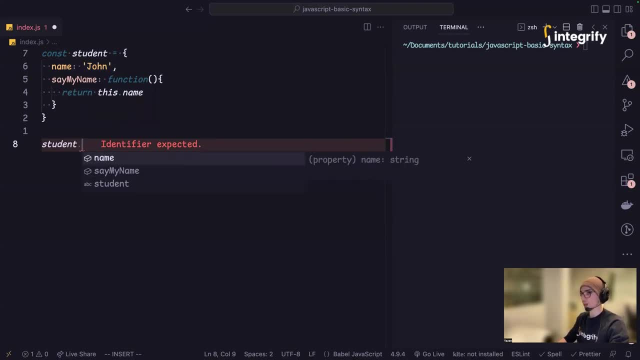 then you could choose either of the available properties you have or by by having this square brackets and inside it you will tell which property you're interested in. so either way, uh, it works like the other way, so, but mostly i'll go with basically the uh, the. 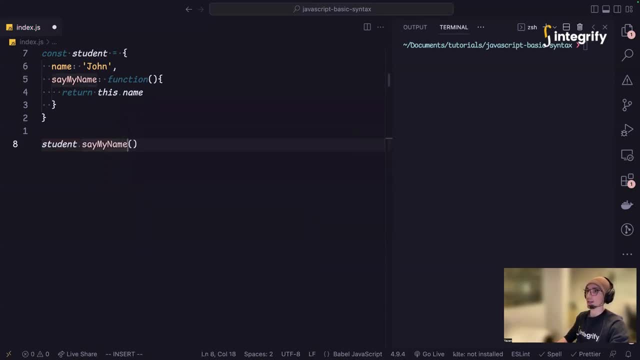 dot uh. so now, because, because, say, my name view is, what is a? uh is a method, so it's a function as well, so i can invoke a function. i'm going to talk about functions in in the moment. so, uh, let's wrap, maybe wrap this into a console log so we can see. we can see the values. 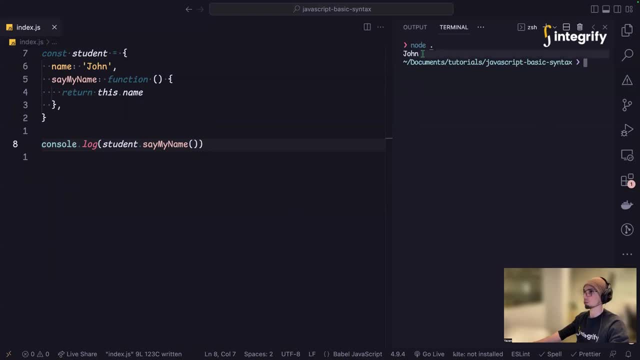 uh, can you run it? yes, here we go now. you can see john here, uh, cool, so. So that's kind of like basically what objects are and what you can do with them. Objects are really fast and you would use it all the time. So, yeah, let's go to the next. 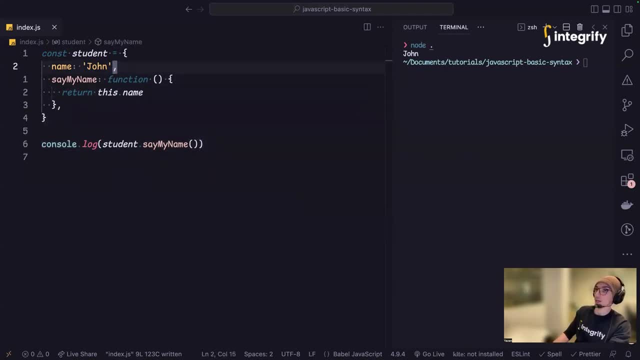 And, by the way, objects are reference types. So, yeah, again, regarding the reference types, I think I will basically just talk about that later, Just to keep this kind of video short as possible. Okay, so, lastly, I think, lastly, we will talk about the or no, we still have functions. 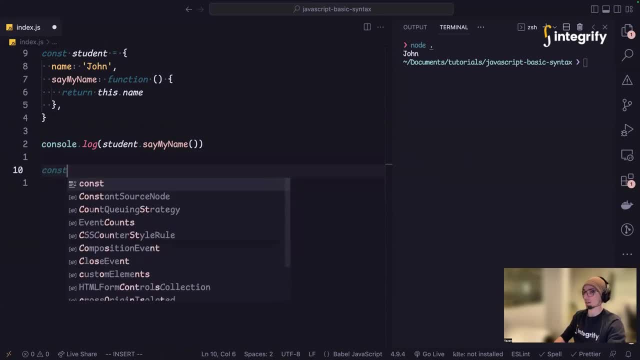 So let's just talk briefly about arrays. So array is also another data structure where you could save a list of, for example, a list of: doesn't matter what, but as long as they have the same type most of the cases- or. 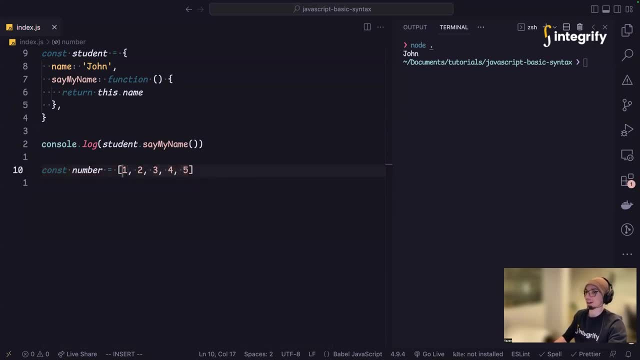 it's better to have the same type right, Otherwise it's going to be really kind of hard to manage. I know we're going to introduce a lot of bugs eventually. So yeah, it's mostly if it's a kind of a collection of a list or a list of the same data types. 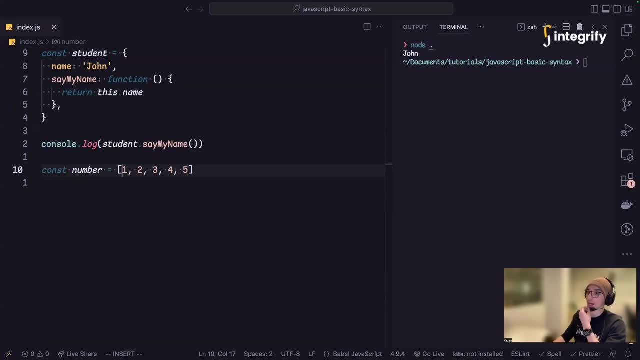 and where you just keep it or store it here, And then what you could do about that. there are so many ways, so many ways to access or to loop through the array and access individual elements. So there's just basically- or this is some numbers because it's a viewer- 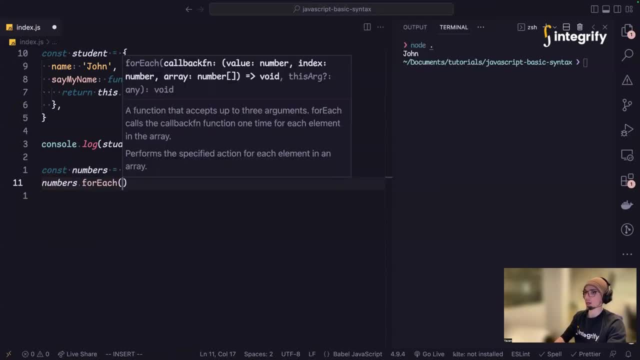 So one of the ways is to use- Okay, And by the way there are, there is like for what I've just talked about. we can just talk for hours and I can explain so many things in details, but I prefer to just for the sake. 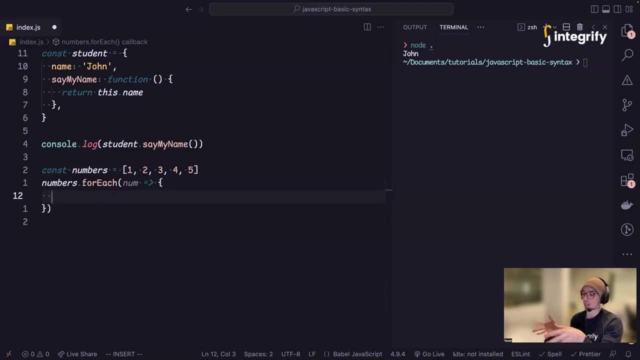 of thinking, to just to keep it short, But if you are really interested to dive deep in in details, into to these stuff and within with more examples and maybe, maybe in a kind of series like like a kind of a series that we first want to talk about, 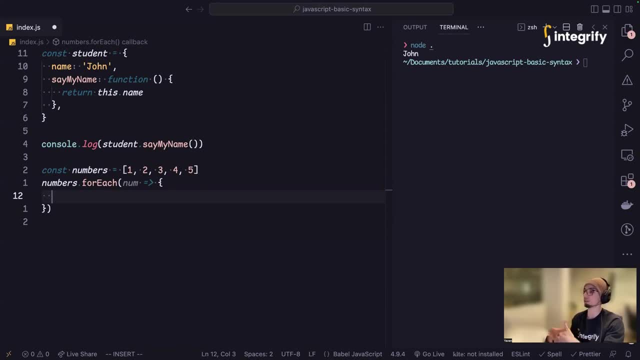 We talk about only functions and then a way, and so on and so forth. So if you are interested, just leave a comment below, So I would know and I could write or prepare something for you in the next videos. So so, as I said, there is one way to look through the arrays which is using before each 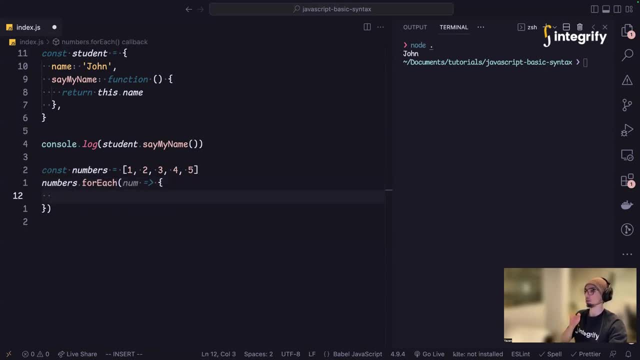 And and and. at this point here, what it's going to do is going to iterate through and every and every array, and you have access. So this is a callback function which basically Gives you access to the, or that's what at least for each method is expecting, right. 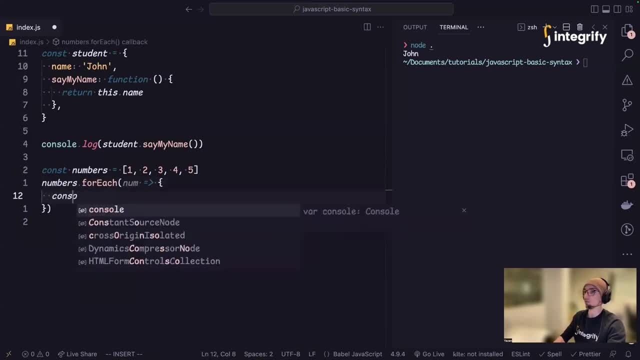 So if you so at this point here in in in this code, if you try to console log num, what we're going to see here is: if I run this code, see you 1, 2, 3, 2, 5.. 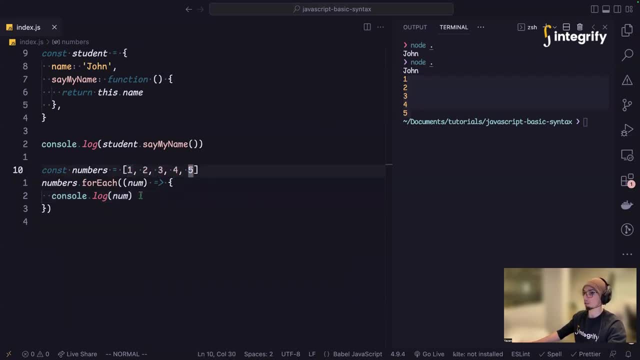 So we have access to every individual and then it's here at every iteration and we can do all sorts of stuff. It doesn't matter, Maybe I want to. I want to multiply those two. So if I run this code, I want to multiply those two. 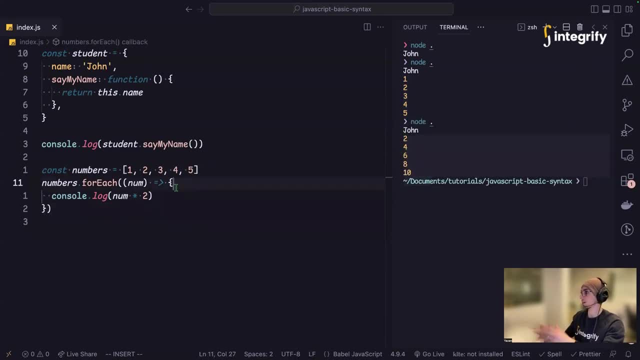 So if I run this code, I want to multiply those two, And again you see that you are multiplying. you know the now the stage is yours. It depends on what we want to do, and so on. But again, there is so much to talk about. 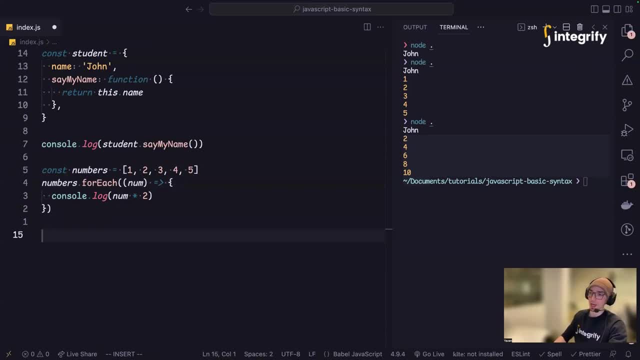 It was just. let me know if you would like to hear more about it. last but not least, is is: is the function, So functions they. the ideal functions is to to do one job. So one task, maybe count or or calculate. 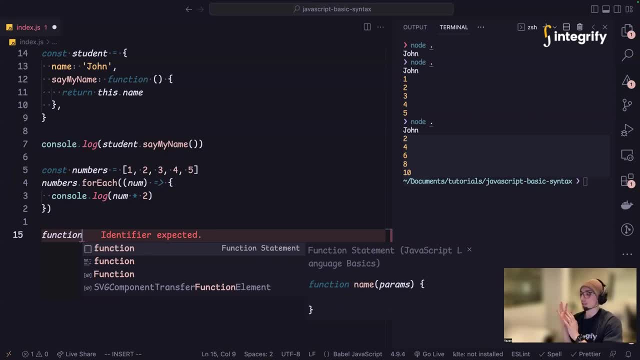 Number numbers, sign in. you know only one specific job that it should do, So let's go with the game. Say My Name. if you guys are freaking bad fans, you will relate to this. So what is the syntax of it? 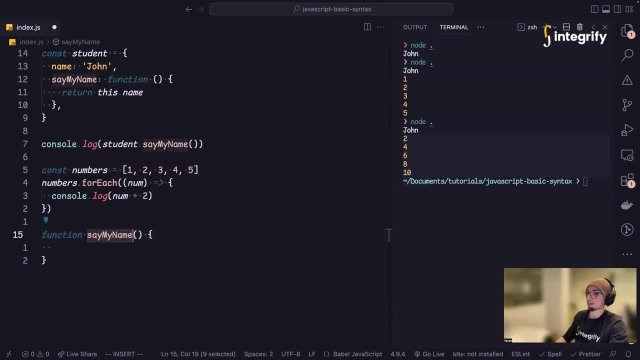 So you start with the function keyword and follow it by the name of the function. What is that function name? It could be anonymous, but it's better for you to have like an actual name word. So here inside the function, you can do whatever piece of code you want to do. 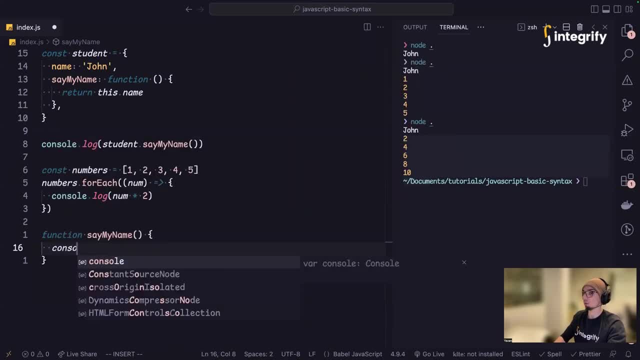 So in this case, here, what I want to have is, for now I'll just consolelog my name, name, So Heisenberg, for example, And if I want to run that specific function, how can I do it? By just saying, say, my name. 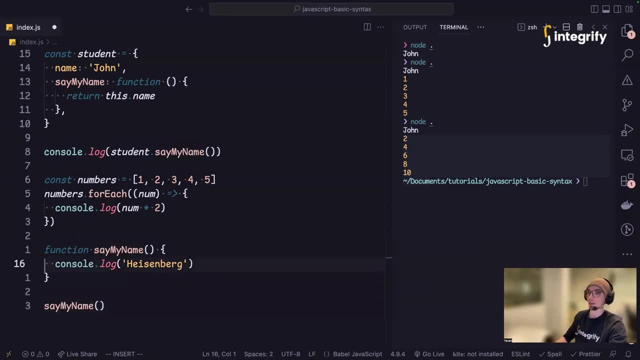 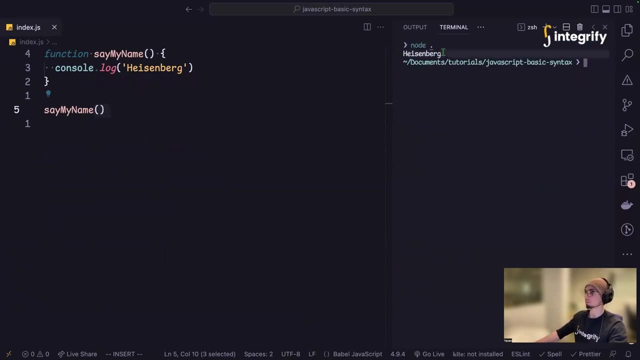 And invoke it. So with these practices I can now just maybe remove all the previous code and just keep this in. So with this process it means I'm invoking the function, I'm running the function, And if I were to run the code here, you could see that it's printing Heisenberg. 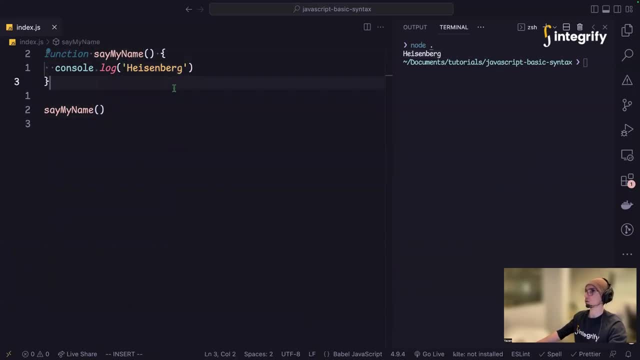 So what if I want to make this a bit more dynamic, right? What if I want to make it dynamic? and it doesn't matter what name I feel it, it just will. it will return for me. for example, Let's just call it Heisenberg. 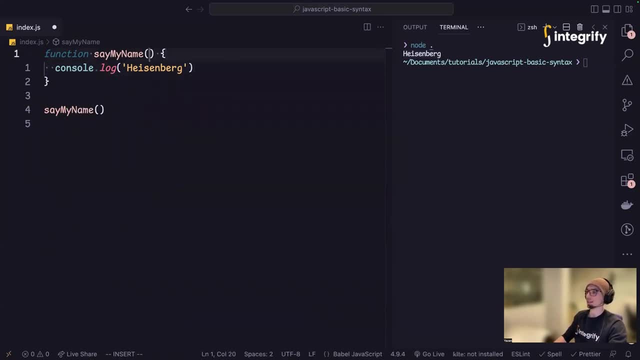 Okay, We will return this again. So in this case, here we can pass stuff or we can pass some data to the function via the arguments. So here I could say I want an argument called name. And now what I can do here- sorry, what I can do- is I can do this, okay, so consolelog. 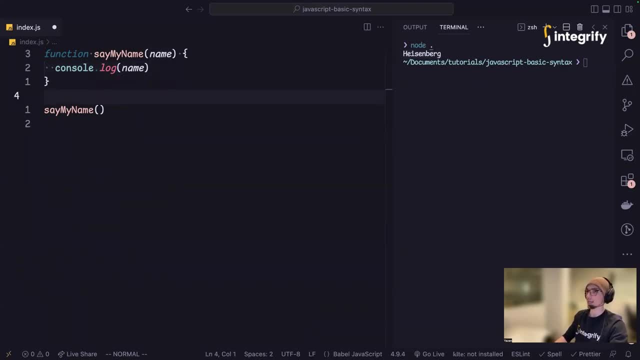 name, for example, And in this case, here when I invoke the function. but for now, if I try to invoke it without actually I'm keeping everything the same. what I'm going to get in this- yes, it's undefined- 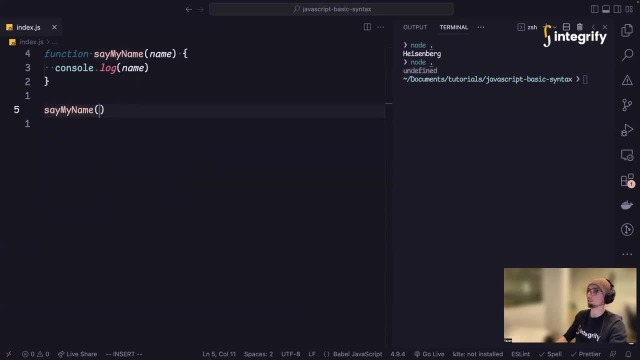 That's great. So because we have not, you know, provided any value here, when we are importing it, then it's going to be undefined because you know it's just. there's nothing there, nothing at all. Remember. 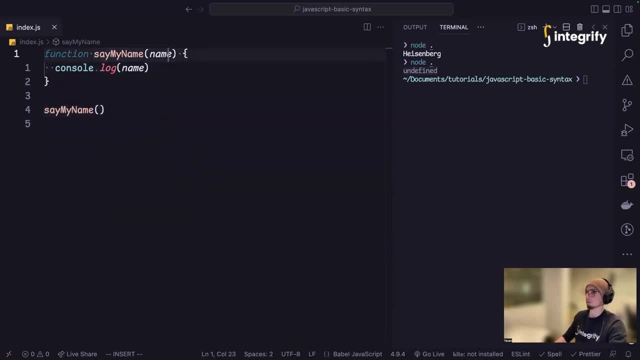 So how can we define? how can we define a variable or a value for the new variable here? So this could be done by by adding a parameters here, or let's, or arguments in this case. So So here we call it. let's just go with, for example, Heisenberg. 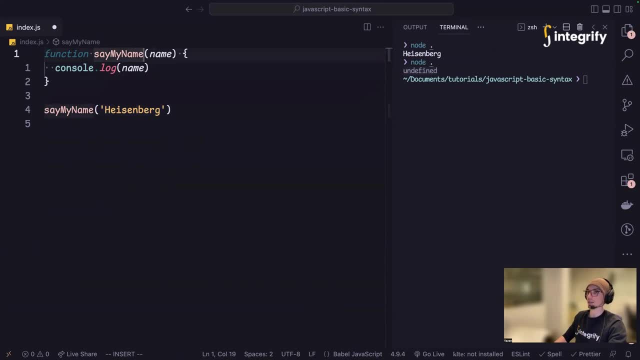 So these are arguments to a function and these called parameters. So we provide an argument here and now. if I would just run that, you see now it's printing Heisenberg- I can basically go ahead and say: okay, let's say my name to John and maybe let's go with. 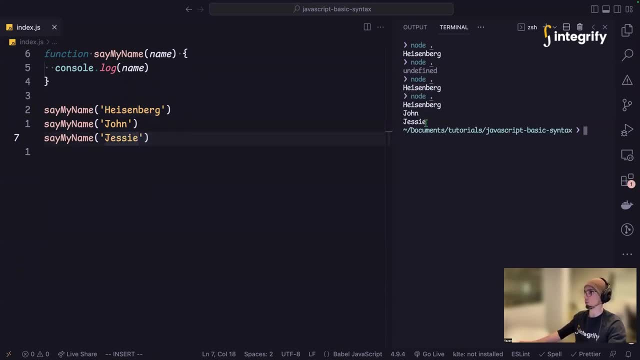 Jesse, for example, And if I run and invoke the functions, now we are basically done, So I can just run that. Okay, So that's basically printing all this tree, The one. one more thing as well, what you could do here you could return value from. 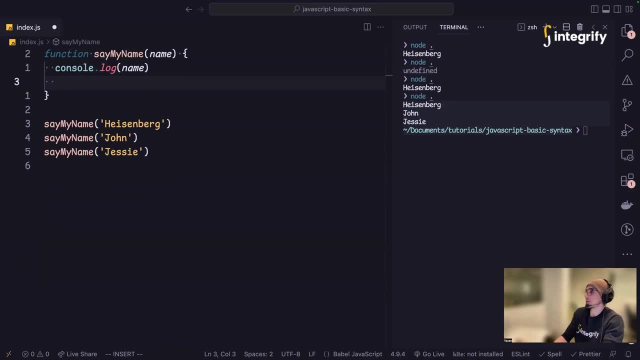 the function. Maybe you don't really. you know reality, don't really. maybe you need to need to kind of console log things. So maybe I would just go with other example. Let's go with a function, maybe, or sum and and the sum what it does. here it takes two. 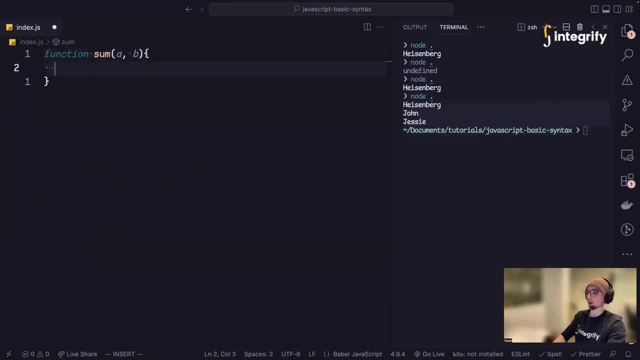 arguments here, So A and B, Okay. So what I'm going to do, I'm going to return this value, So A plus B, And so when I'm invoking it, I just say sum and then remember the order matters. 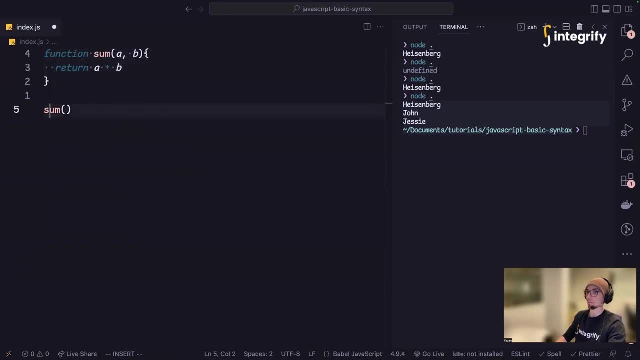 So if this is at the beginning, then this is the first and that's the second. So sum two and two. So what's going to happen here is this: data from this argument will go all the way to these parameters and then travel to this line. 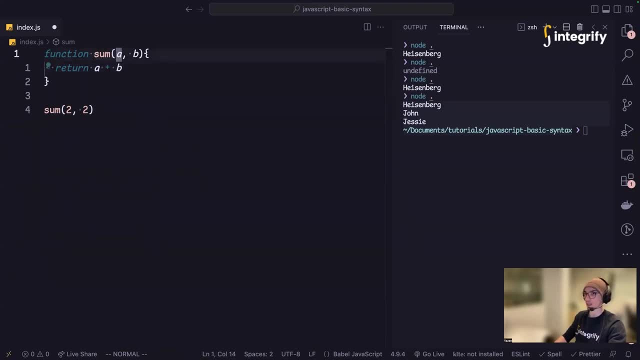 And then the computation will happen, which is A plus B, So two plus two. And if I try to kind of like now, I need to console log it, because at the moment it's just returning. I'm not doing anything with it. 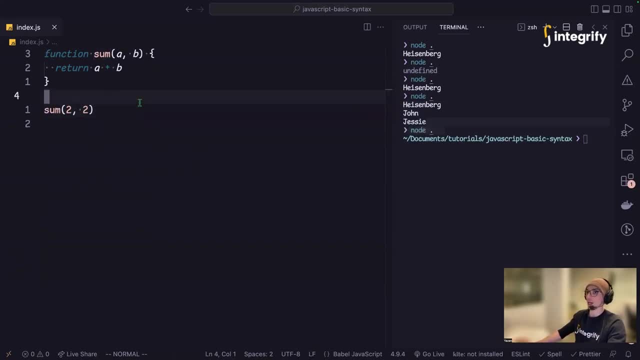 Like if I would do node or run it, you see it's just empty. I could maybe just basically just go ahead and and assign it to a variable, Like I would call it I don't know out of, out of out of ideas, I don't know- final. 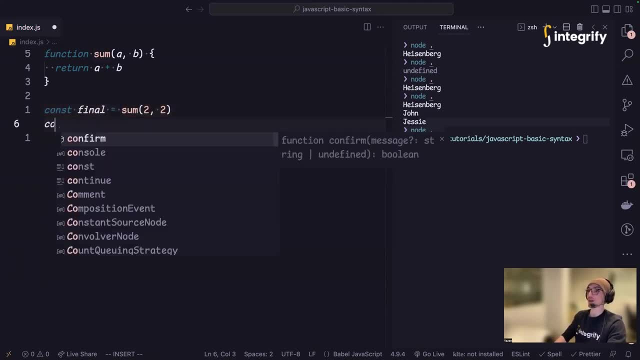 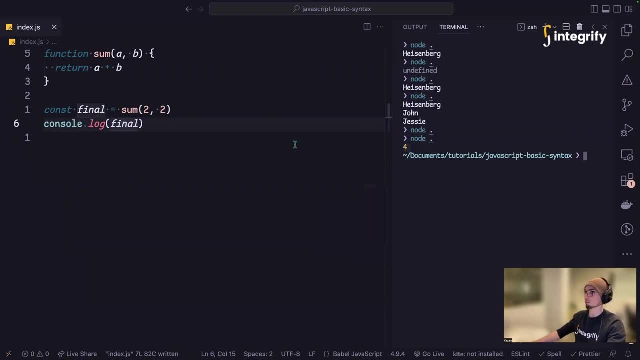 And let's do that, And if I do so, And if I do so, And if I do so, And then if I do and run the program again, you see now it's printing for. And then if I do and run the program again, you see now it's printing for.